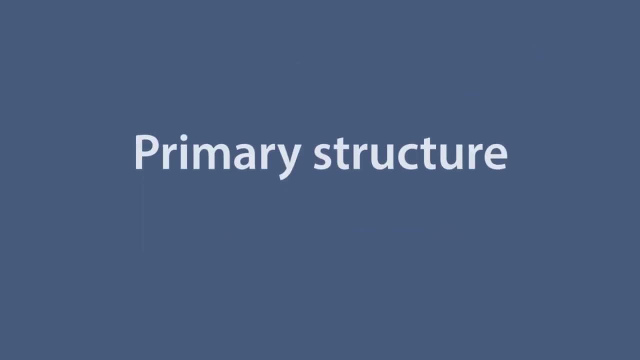 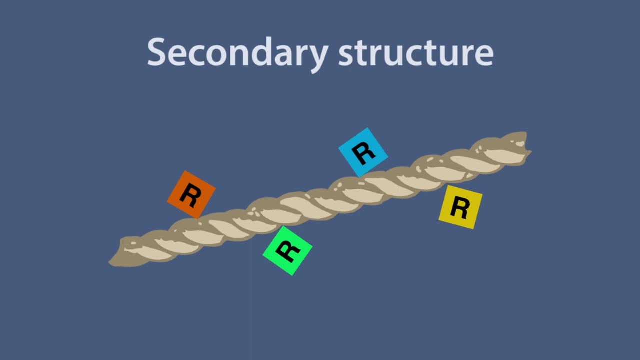 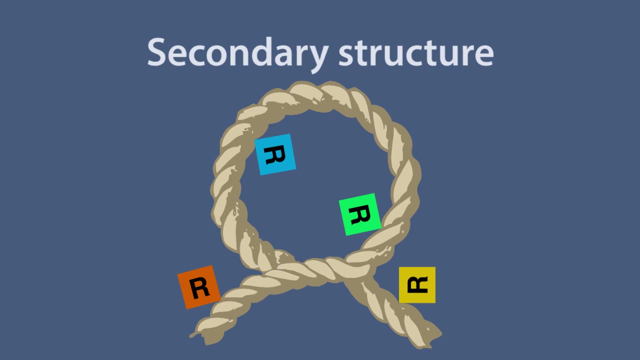 into our own proteins. Enzymes have a primary structure, which is simply the polypeptide chain. we have just seen The secondary structure enables the protein to coil up like a twisted rope. Now the different side chains attached to each amino acid, represented by the different colored R's: 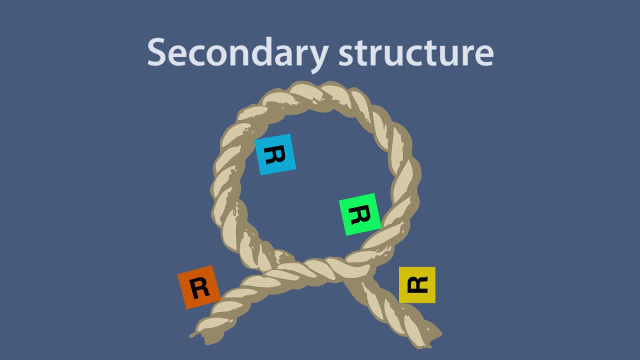 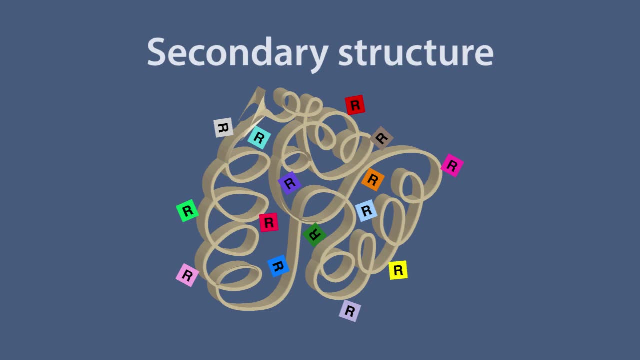 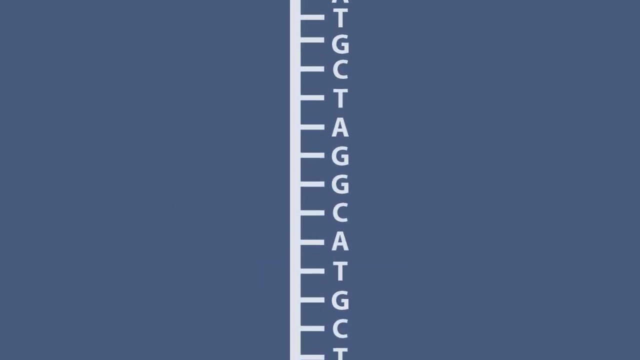 stick out like bits of rag caught in the rope. Some of these will attract each other and some will not, enabling the rope, our protein, to coil up in a very specific 3D shape, giving it its tertiary structure. Here's how it works: The genetic code of living things, safely stored as 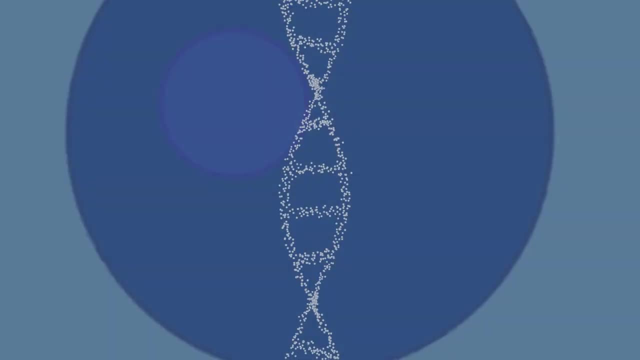 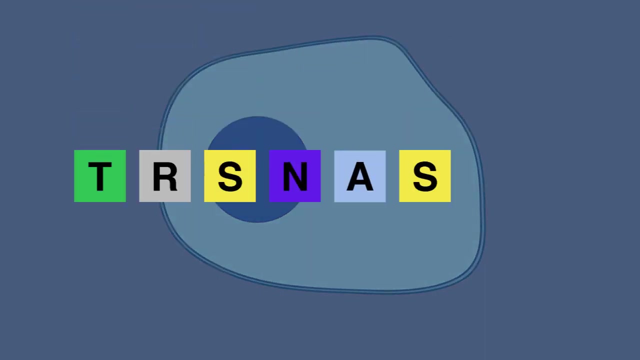 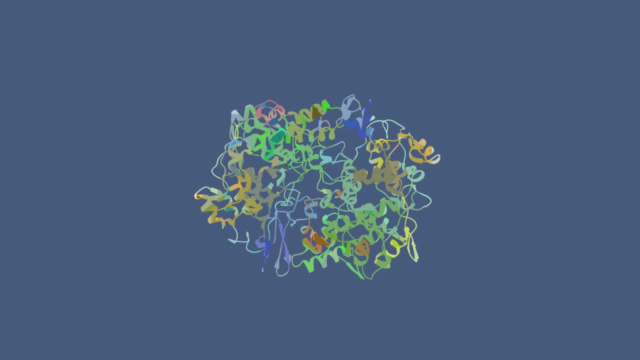 DNA on the chromosomes in the nucleus of cells sends out a coded message telling the cell to construct a protein made of amino acids joined together in a unique order. This coils up into its final 3D shape, ready to catalyze one type of reaction needed by the cell. 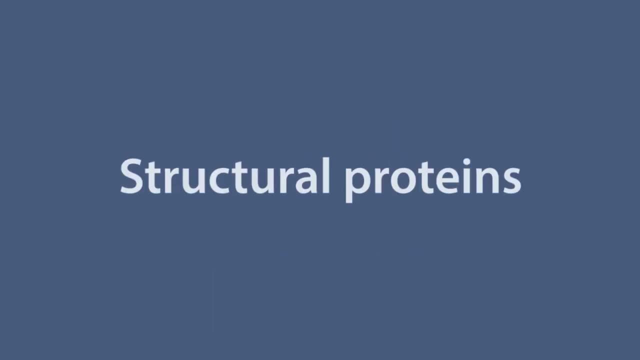 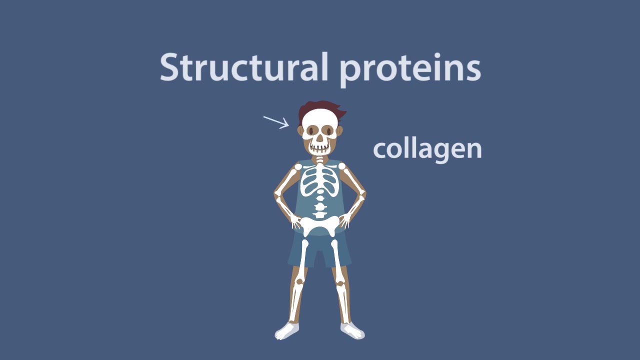 A bit about the structural proteins that build the bodies of animals such as worms, insects, birds, fish and ourselves. Our biggest organ is our skin, made of tough protein. Bones are made from a flexible tough protein called collagen- Try feeling your ears- Then calcium phosphate. 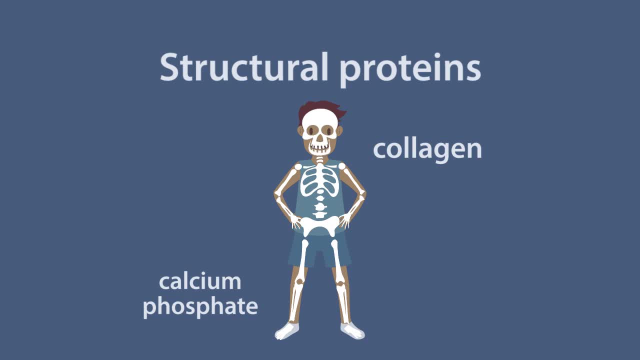 a hard brittle, insoluble salt is laid down, making the bone a bit like reinforced concrete. with the tough, flexible collagen fibers like steel and the hard brittle cement around them, Protein molecules in muscles are spread out and they contract. 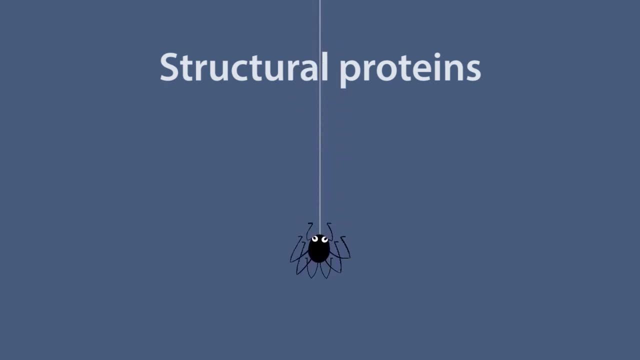 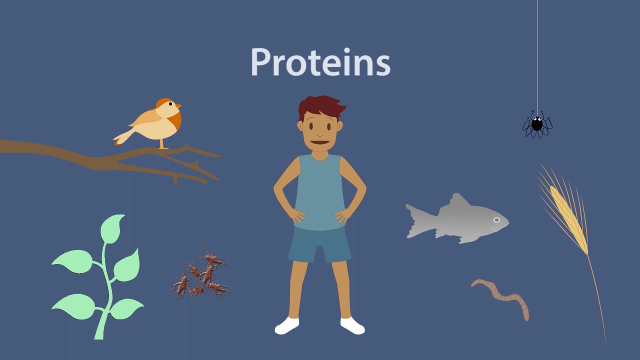 when activated Spiders and some insects make threads out of protein. They are very strong and tough, but soft. So, to summarize, we learned that proteins are vital to all living things, since they are the enzymes that control all the chemical reactions in their cells. In addition, 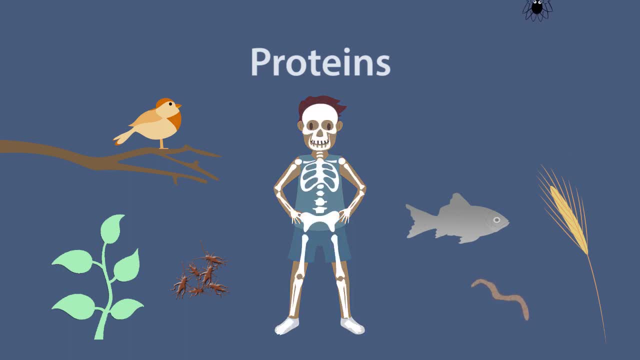 animals use protein to build their vital organs. Digestion breaks the protein we eat in the body and the cells in the body are the ones that control the chemical reactions. Digestion breaks the protein we eat in the body and the cells in the body are the ones that control. 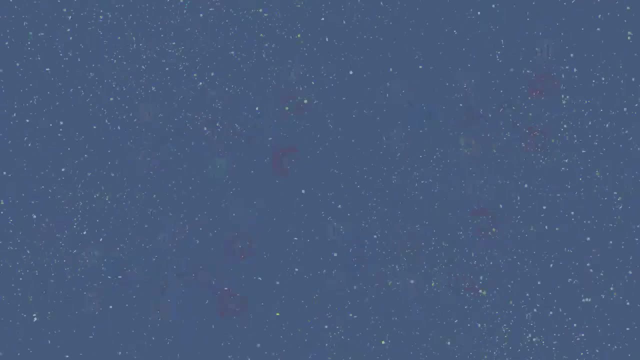 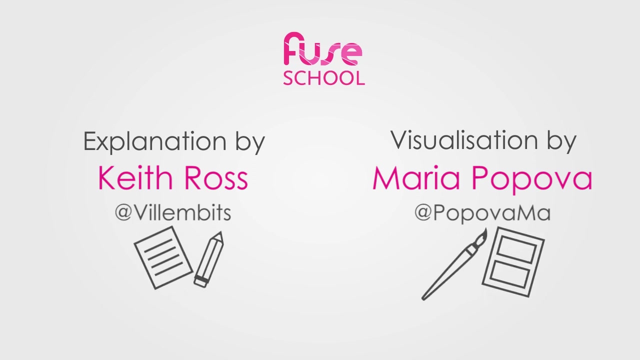 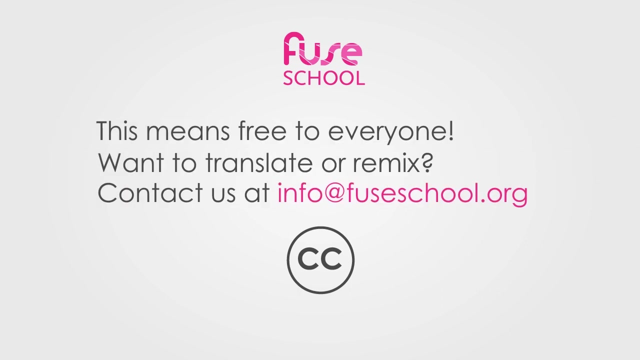 the chemical reactions, Digestion breaks the protein we eat in the body. DESIGNATIVE COMP Riviera: The you.